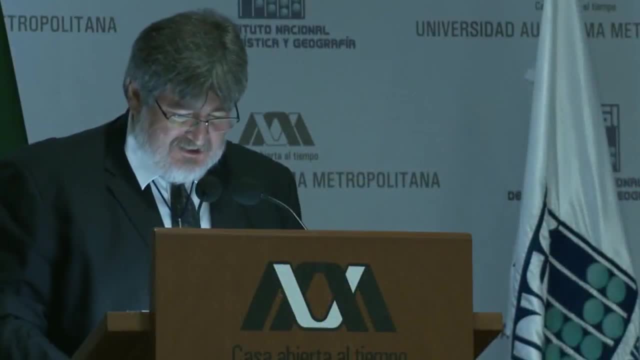 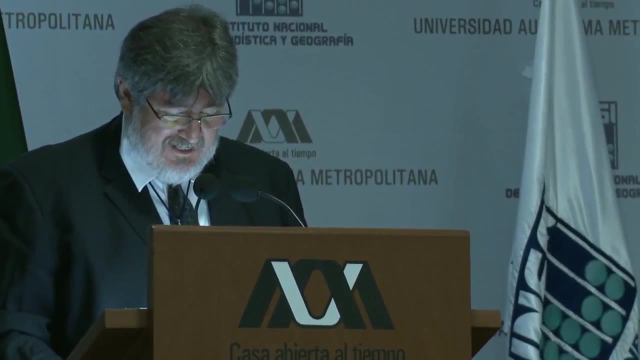 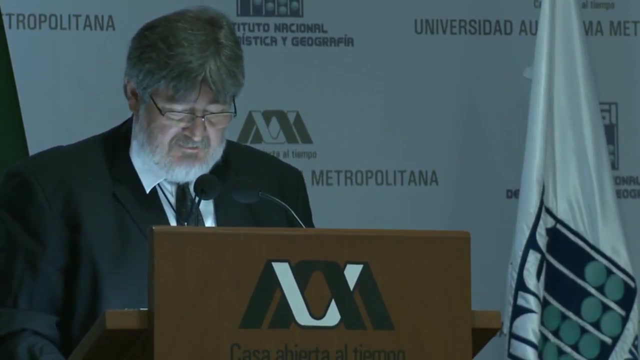 Now we will continue with a presentation of Javier Aparicio-Mijares, who started the School of Engineering from the UNAM and graduated with a Master's in Hydraulic Engineering in 82 and in 85, PhD in Hydraulic Engineering with a distinction in the same division of Postgraduate Studies of the School of Engineering. 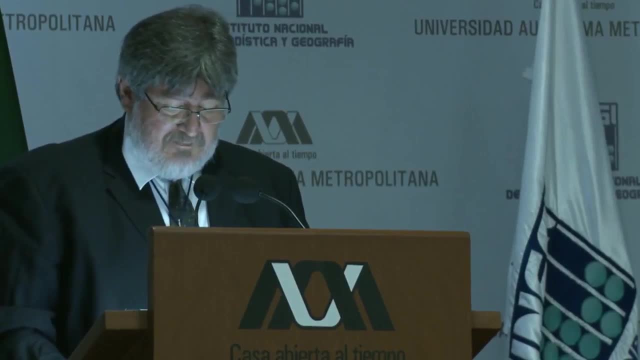 Within the Mexican Institute of Water Technology, he has been a specialist in hydraulics and coordinator of hydrology, a position he has right now. Dr Aparicio has a full trajectory in Postgraduate Studies and is the author of books. He has also published 118 articles and has received the Enzo Levy Award in 2004.. 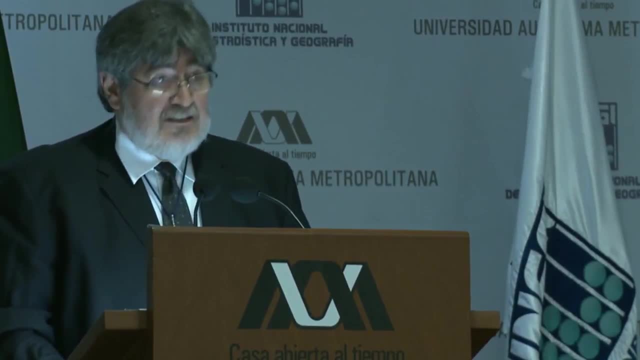 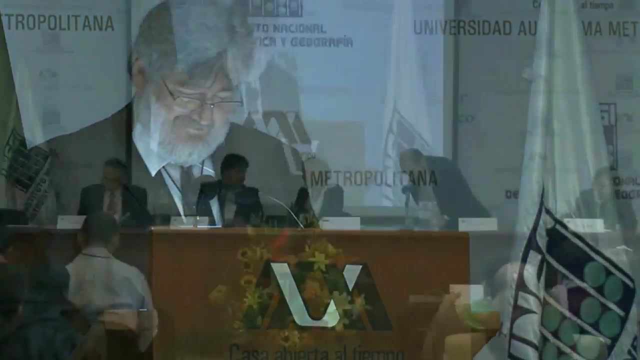 And he is a member of the Mexican Institute of Water Technology. Dr Aparicio is also the director of the Mexican Hydraulic Association and the National Researchers System. His presentation is on analysis and hydrological modeling of the quality of water in trans-border areas between Mexico and the United States. 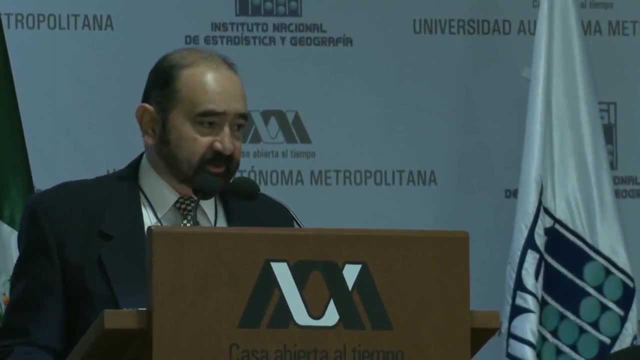 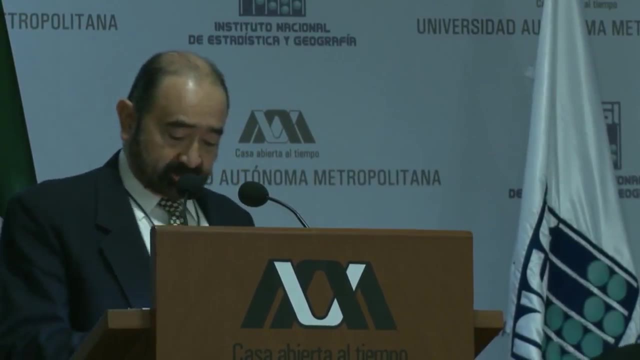 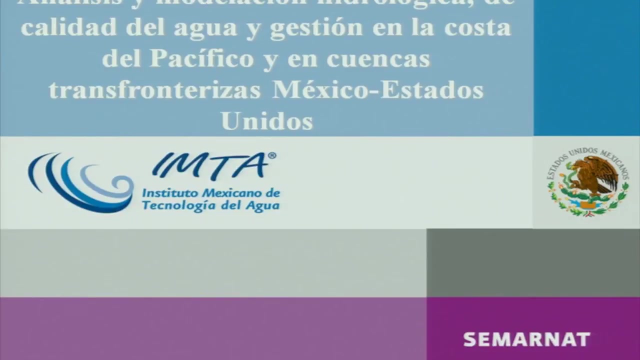 Good afternoon to you all. In the first place, I want to thank the invitation extended to us by the UAM and INEGI to participate in this meeting. Well, will you please put it on the screen. I will talk about some work of the Mexican Institute. 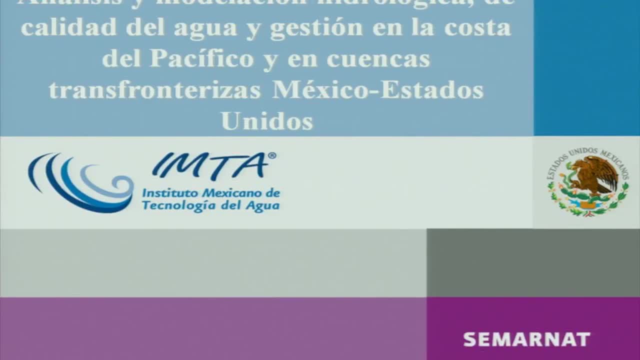 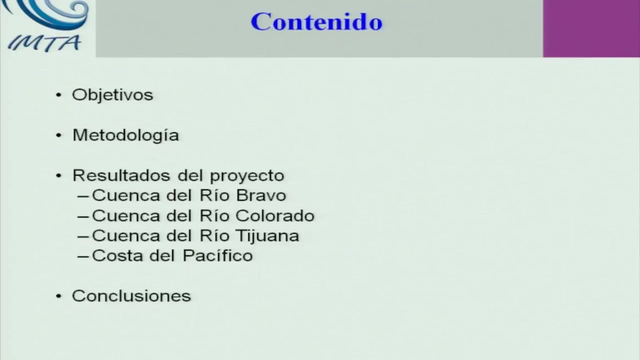 for Water Technology Analysis and Hydrological Modeling, the quality of water, management of water in the Pacific coastline and trans-border basins between Mexico and the United States. Well, first I will introduce the goals of my talk, methodology of goals and results in the basins of the Rio Grande. 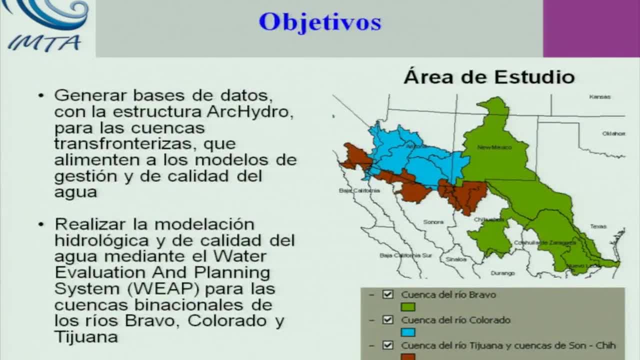 Colorado River, Tijuana River. The goal is to produce databases, personally, with an specific purpose, With an specific structure, which is ARC, Hydro for trans-border basins, And make these database and the models on the quality of water. and the main goal is to compile all the geographic information systems. 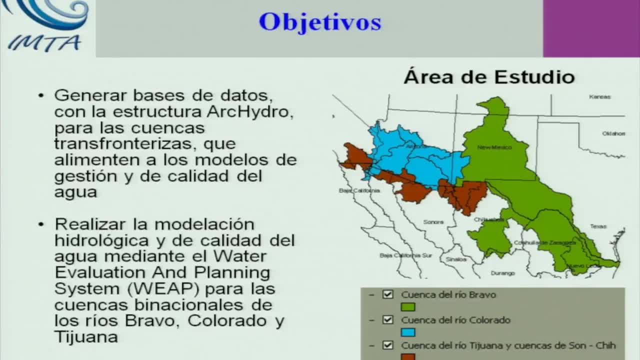 with these management models so that the management of water is more efficient in this hydrological model. Thank you very much. Thank you, And the management models are carried out through WIP Water Evaluation and Planning System that was used for these water basins. 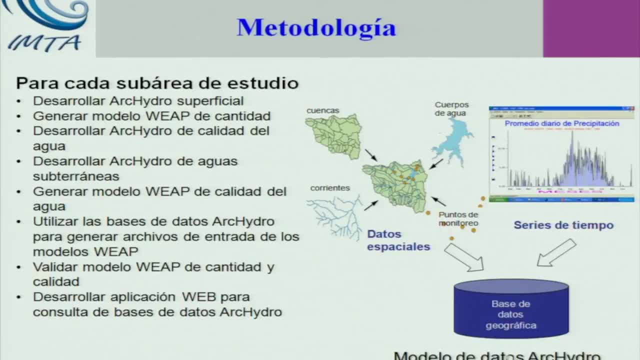 For every sub-area, basin and sub-basin, we have developed an information system on the surface and then we create, create a WIP Model for the amount of water, For the amount of water, Then we develop again the Ar-CAREDO and the Acrohydro. 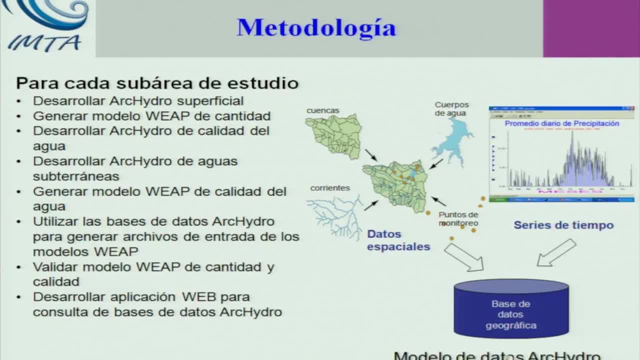 and then the WIP, and then we validate the models And then we come up with the applications. And the Ar-CAREDO data model is a model that takes into account the status, characteristics of the information, such as the basins, the bodies of water, the streams, the spatial data, the 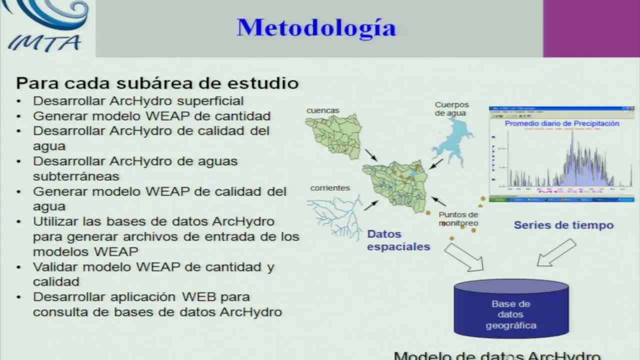 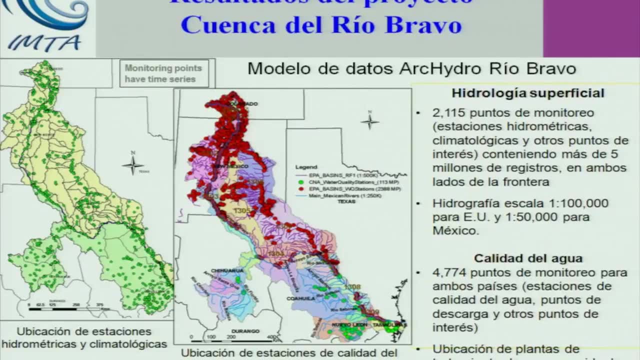 temporary data, the seasonalities, the seasonal data, rainfalls, droughts and so on and so forth, and all of this and the runoffs, and, in the case of the Rio Grande, we have here the location of the hydrometric and climatological stations. 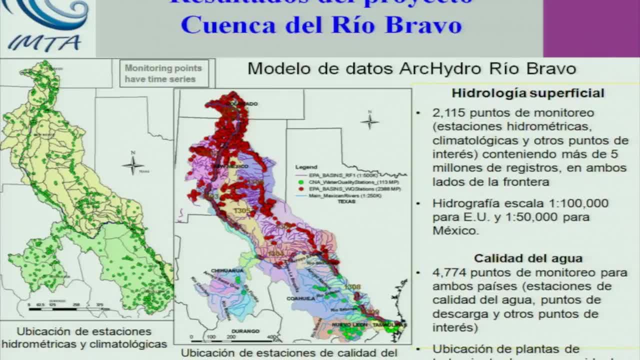 and we find here the stations that have been put to use. Now it so happens that when we look at the maps with information on Mexico after the Rio Grande and going up north, the maps are blank, And vice versa when we look at US maps, where we need information on the Mexican 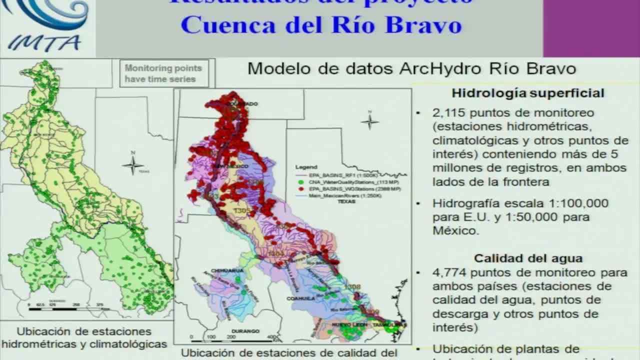 side, on the south of the Rio Grande, maps are blank, and one of the goals we have here for this work is to come up with an integral system that will include all the existing information on the side of the United States and Mexico in regard to the international basins and for surface hydrology. we have to over 2,000. 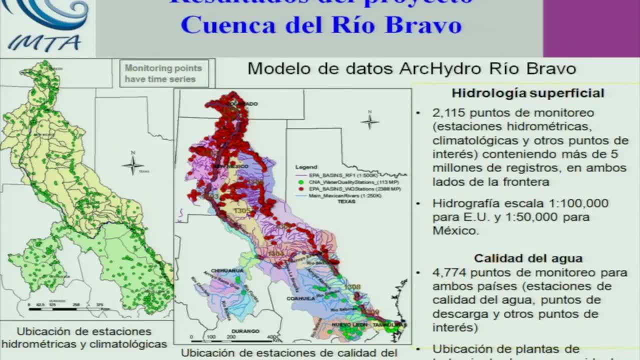 monitoring points, A climatological hydrometric stations with over 5 million registries on both sides of the border, and this is an effort that has that is totally unprecedented in regard to compiling all the information and being able to plan the management of water in a joint manner between the two countries and in 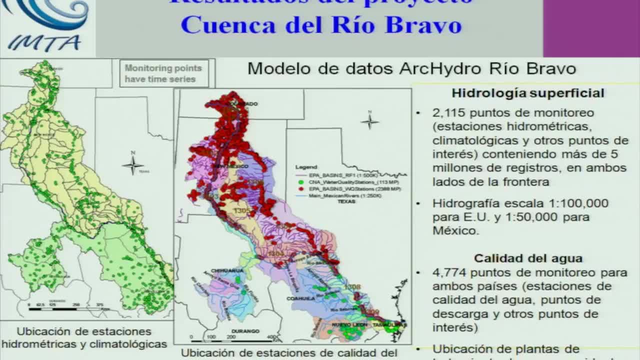 regard to the international basins. In the case of the hydrography, the information for the US and the United States is very important. The US has been 있어 quizcase en el 13 de loESSI, en el 20 de agosto de 2016. 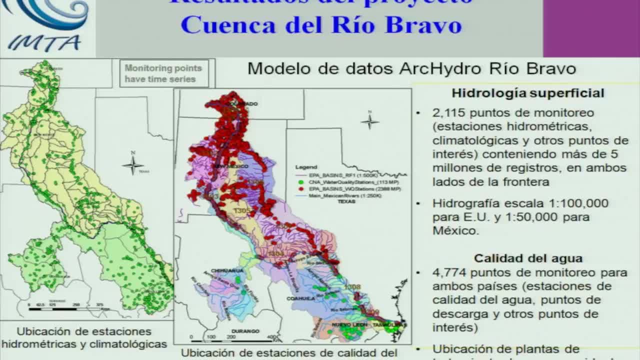 por el Distrito General de laws para escuchar y decir que una vida al despo individually. el 6 de mayo de 2017, nadie espera una health expert sobre diferentes partes del reino colombiano. Number two wall water for both sides of the border at the sea and sea and Mexico is one 50,000 in the case, The age of the quality of water. we have here the map of the stations monitoring the quality of water on the board sides of the of the border. in the US We have a lot, many more stations, and Mexico, but all the monitoring sites when this work was carried out for the monitoring of water for both countries: over 4,000 points of monitoring of water for both countries, over four thousand points of monitoring. 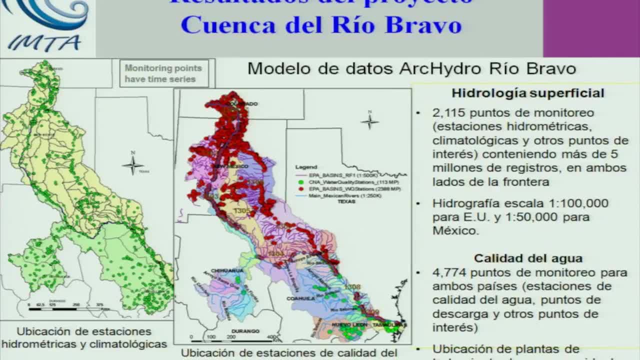 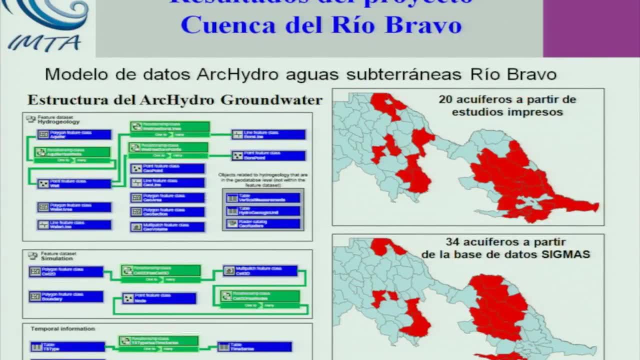 monitoring points for both countries, as well as a residual treatment plants or residual water treatment plants. now, in regard to the archive data models, in the case of the Rio Grande, we have the arch hydro for ground waters and we need information of 20 aquifers based on the survey, 74 aquifers based on the data. 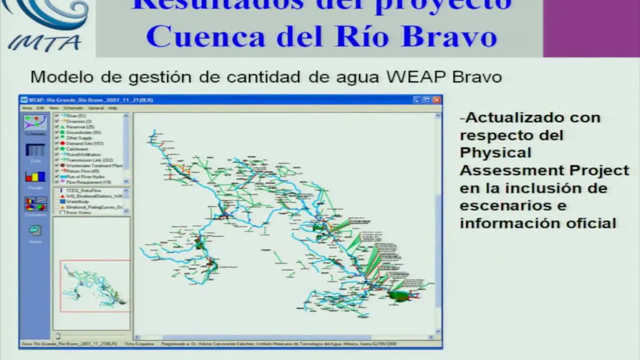 provided by Konawa and for the management model in regard to the amounts of water that we up a whip. we Bravo one of the screens we have for the web models in regard to the volumes of water, the amounts of water, and, in principle, we used a binational project called the physical assessment project. 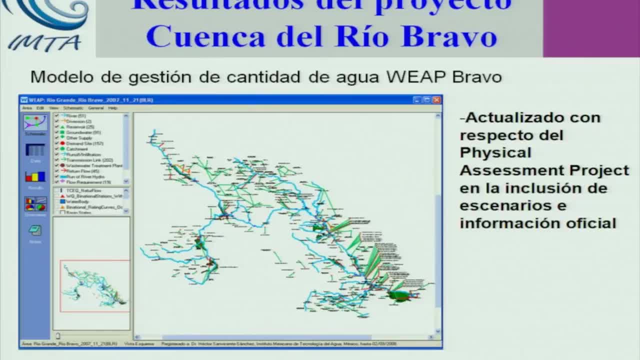 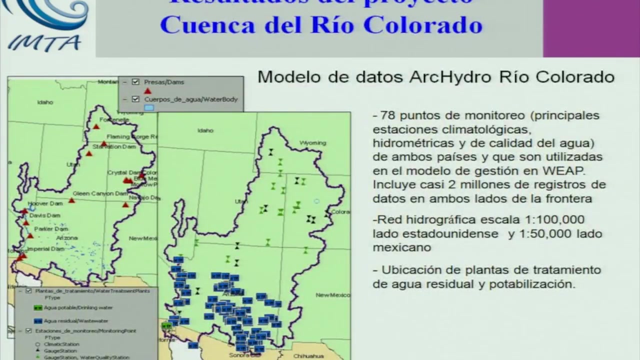 project that tried to assess them, to try to assess many proposals for the management of water in the Rio Grande a basin, but this cannot be modified for different purposes in projects for the management of water at a binational level. in the case of the basin of the Colorado River in the you in in the US. 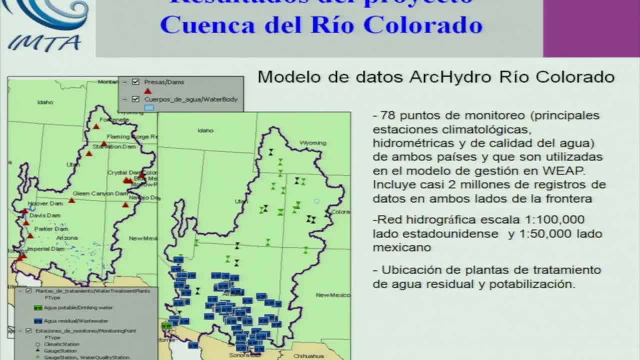 well, most part of the basin is in the US and a small part is in Mexico, but in regard to the water limitation provisions dating from the 1944, Mexico needs over a billion cubic meters of water. that reached the border here between the US and Mexico and we have had many historical events and we are 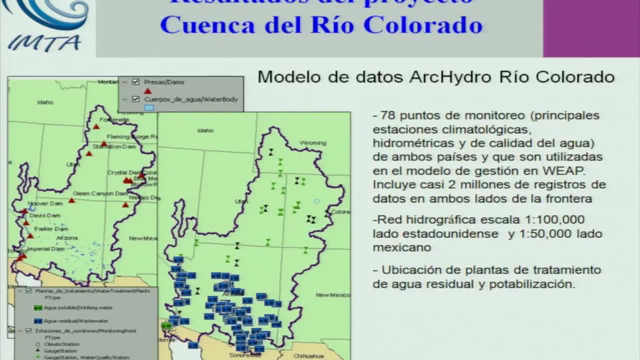 there has been disputes between the US and Mexico because of the quality of water, because of the brackishness of water, and Mexico's part of the fact that they have a fragment of the basin is still an important factor in the management of the basin and in the Rio Grande we have 78 monitoring points. 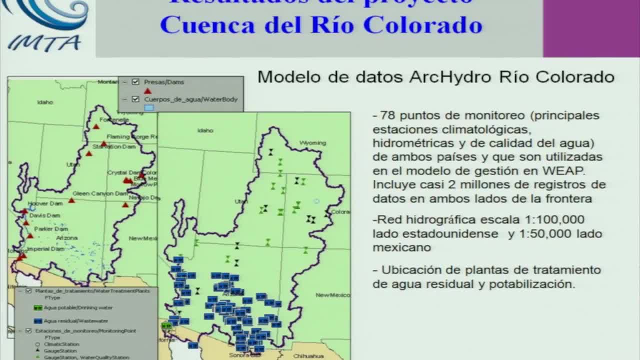 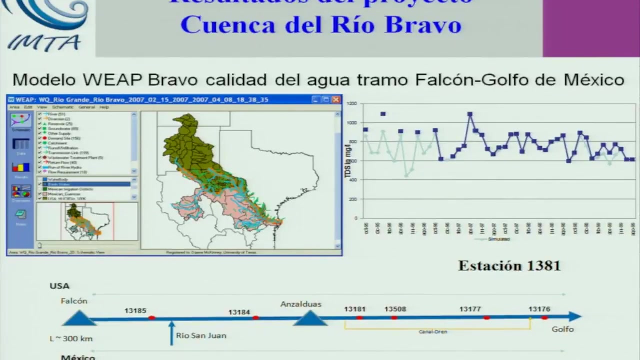 inside the climatological hydrometric stations on both countries. and of course we have the. we have here some examples of the weep entries and exits for the quality of water from Falcon to the Gulf of Mexico, that's straight from the Caribbean, from the Paseo Caracol to the Apaque. 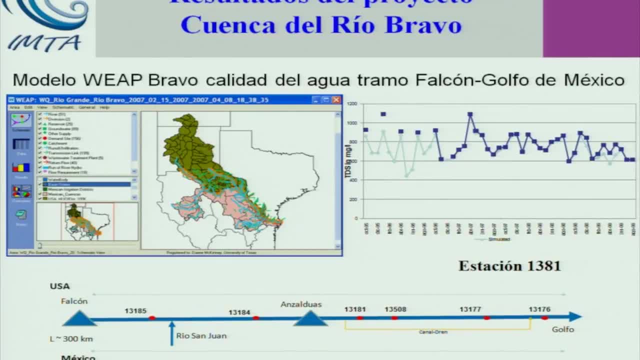 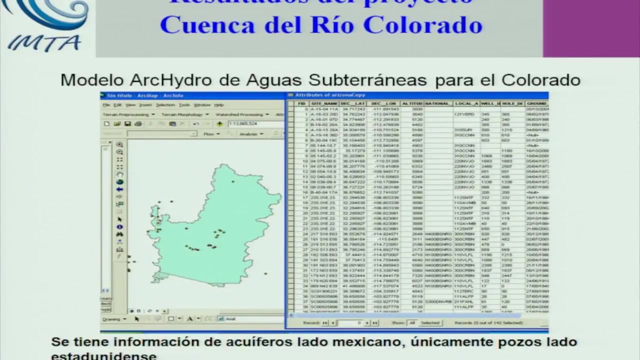 That stretch. we see the variations of the total solids in a station on that stretch and the location of the stations that we have between the Falcon Dam and the delta, the estuary of the river to the Gulf of Mexico, And we have here the archhidro model for the Colorado River. 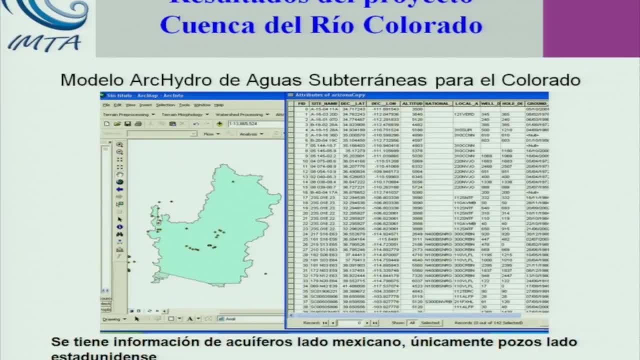 and the Mexican side. In the US we only have information about the wells And this is due to the way the information is managed and handled and the way the water is managed in the US side, different from the way water is managed in the. 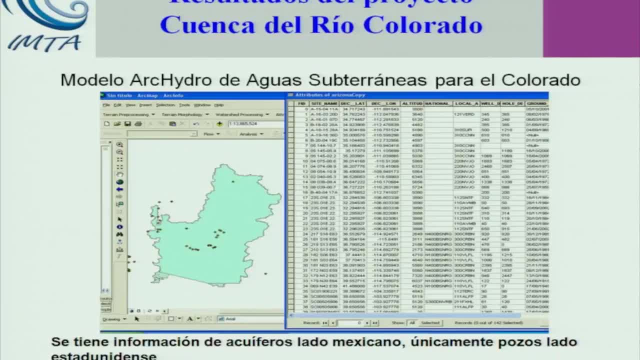 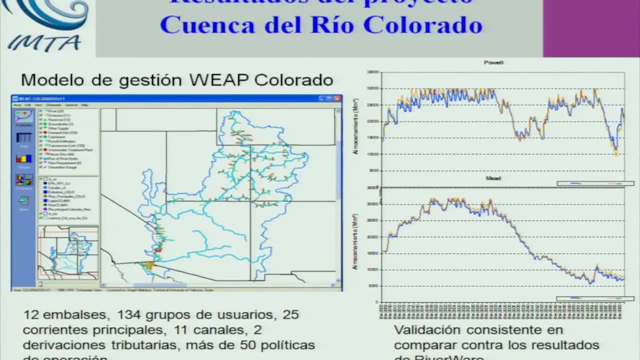 Mexico And on the Mexican side. on that side the aquifers are private and it is hard to have official information. So some of the outcomes from the WIP management system for the Colorado River and we are currently using information on two reservoirs and the channels and the streams and some 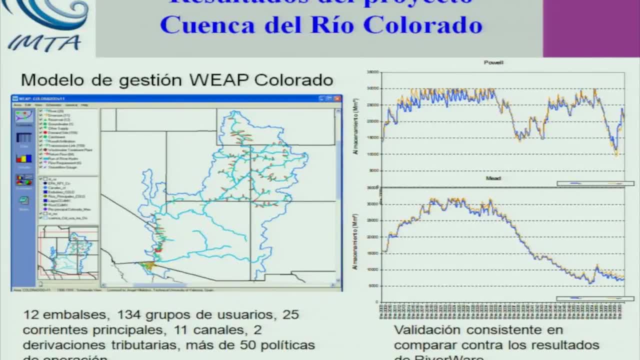 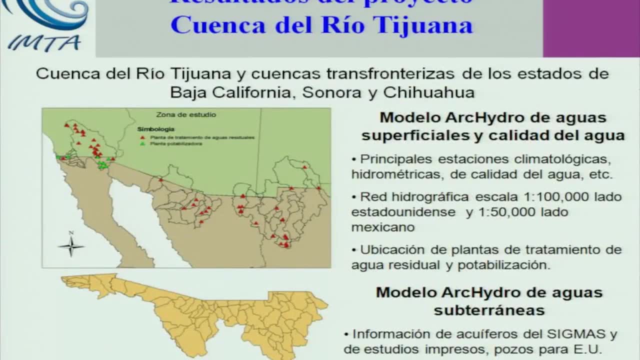 operations policies And I insist, they can be modified at any time in order to be able to evaluate, And we will evaluate them in the model Now in the case of the Tijuana River. this is a stretch of the Tijuana River that comprises many cross-border basins, Baja. 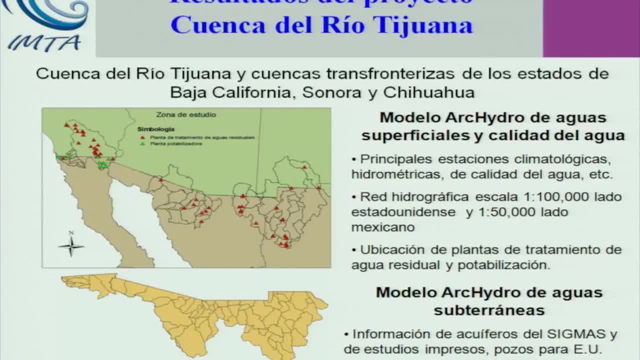 Sonora and Chihuahua in the Tijuana Basin, and there are other watersheds that are here. They don't belong to the Colorado River, nor the Rio Grande, nor the Tijuana River, and that also englobes the information. 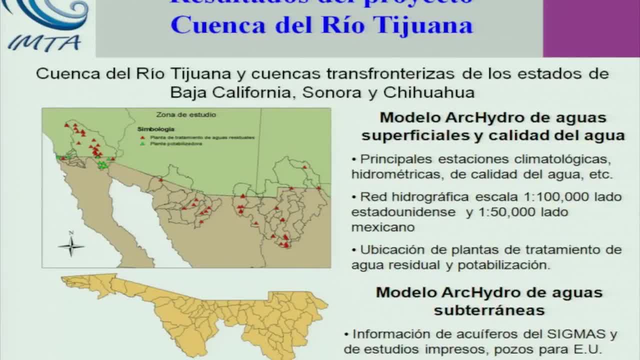 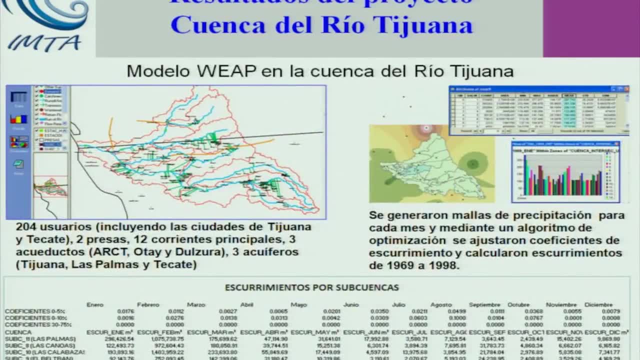 So this is an example for the surface waters quality of water in all these basins, as you can see here in the picture, And here, for instance, we have some results of the WIP model in the basin of the Tijuana River, 204 users, including the. 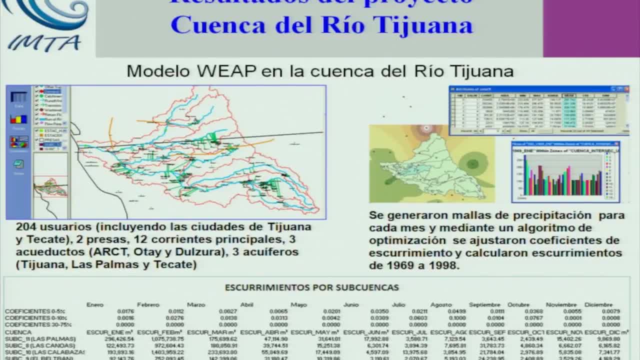 cities of Tijuana and Tecate, two dams, three aqueducts, three aquifers And here, amongst many other things- and this is performed in the other basins- the levels of rainfall and optimization algorithm, and we calculate the runoffs in whatever season we. 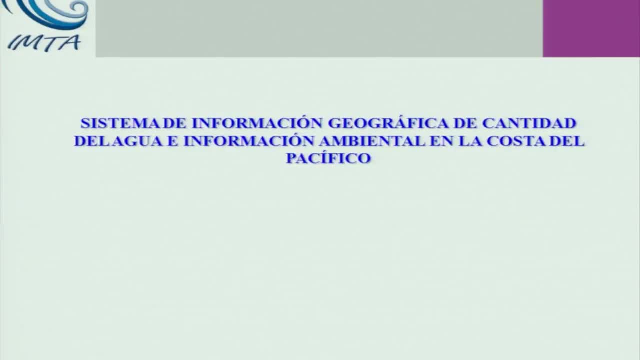 choose. Okay, Now that for the cross-border basins- Mexico, US- and we have applied exactly the same methodology to many other sites around the world. We have done a lot of research around the country. Recently, we worked on a geographical information system. 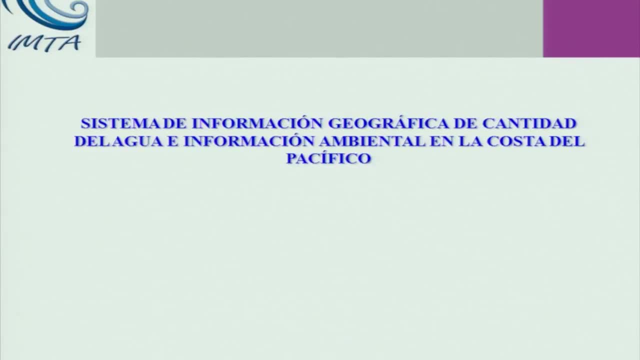 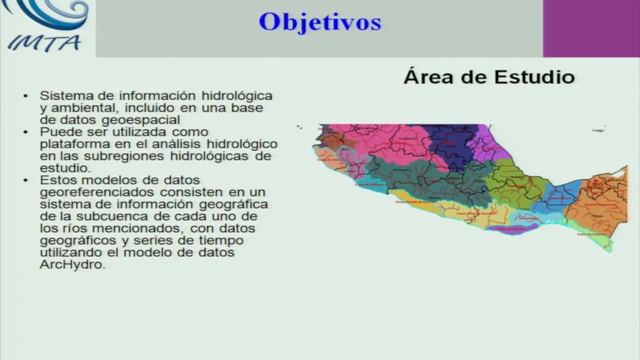 in regard to the quantities, the volumes of water and the environmental information in many basins in the Pacific shores, the coastal line of the Pacific, And here we need to develop an environmental and hydrological database. They are hydro And that can be used as a platform for hydrological 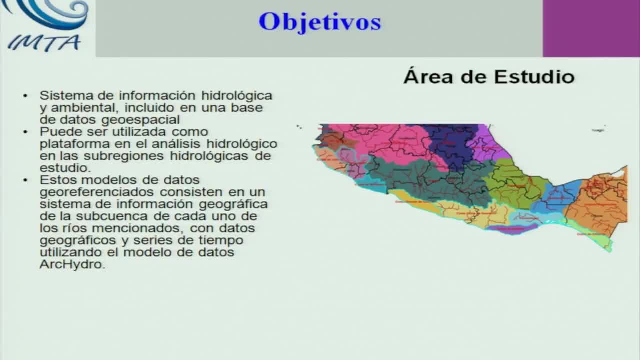 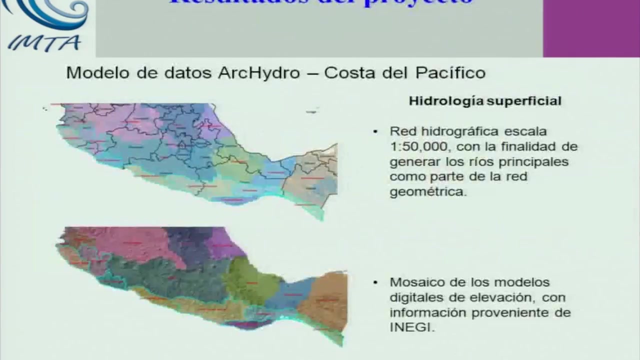 information in these subregions And here, in light blue, we see the basins that were surveyed, that were utilized for this study. Now, these models of reference data, geographical information on every subbasin, the sets of time and rivers, as I said, with the 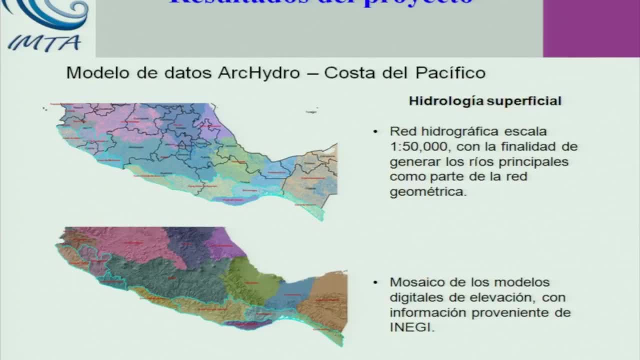 cross-border basins. that's the way that we did it too. Now here we have another example of what comes out from the data model: the hydrology, surface hydrology, the hydrographic network, the water network, the main networks as part of the 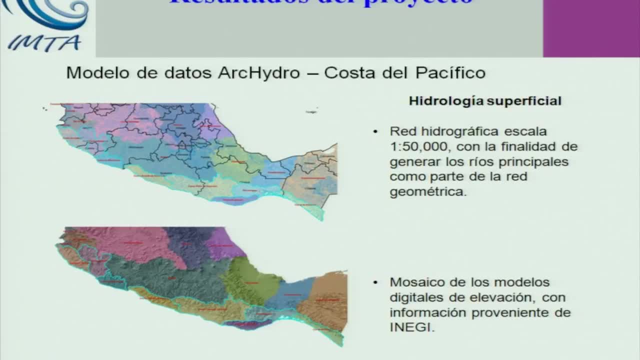 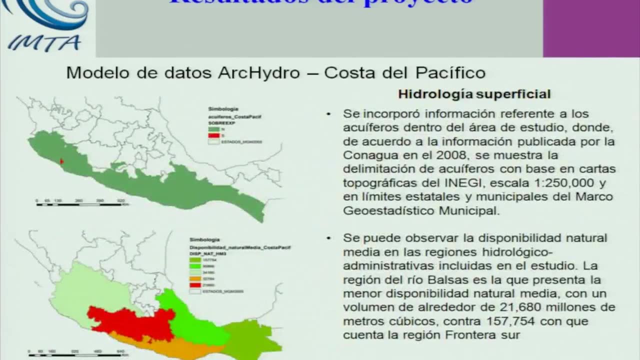 geometrical network and the mosaic of digital models, elevation models, of course, with information from INEGI, And here we see part of the surface hydrology, with the information of aquifers, the area of the study, And we find the delimitation of the aquifers in regard to the 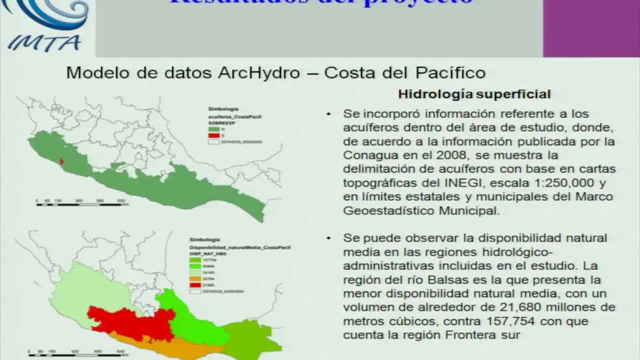 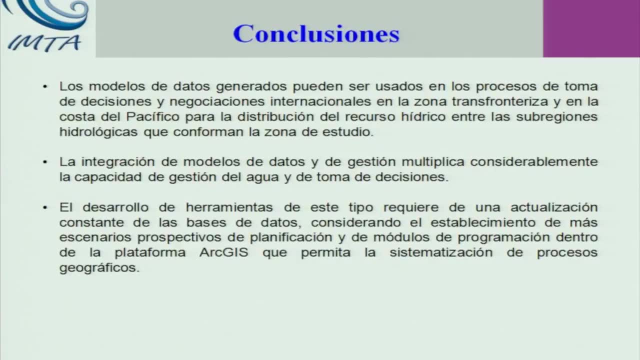 maps of INEGI 1 to 50,000, municipal and state maps and the feasibility we have in many regions. And then my conclusion. The moderator will see that I took more time than was planned, but three exactly. The data that were produced can be used in the decision-making.